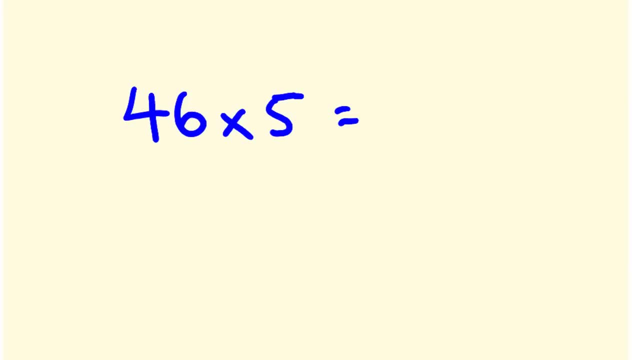 So the way that I'd work this out, the method I'm going to show you, I'm going to launch into it straight away- is what we do is we halve this number here that we're multiplying by 5. So half of 45.. 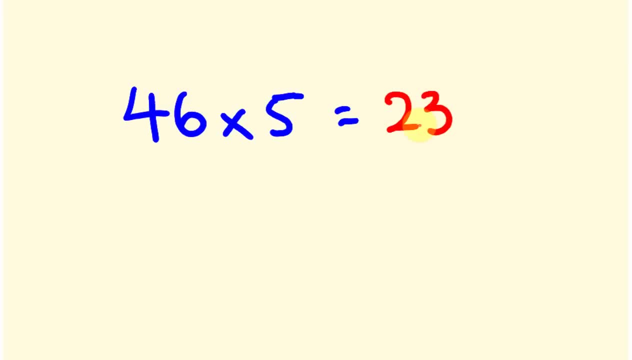 Half of 46 is 23.. Then we just multiply our answer by 10. We just put a 0 on the end, So 230.. That's how easy this is right. Okay. so what we did is we halved our number and we just put a 0 on the end. 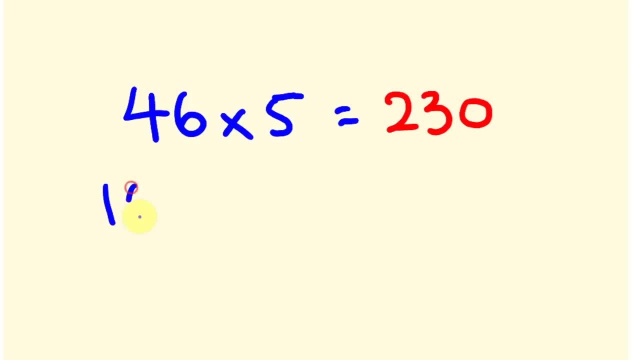 What about another one of these? What if you got asked the question 106 times 5?? So same sort of thing. We're going to halve our number, half of 106, which is 53. And we put a 0 on the end. 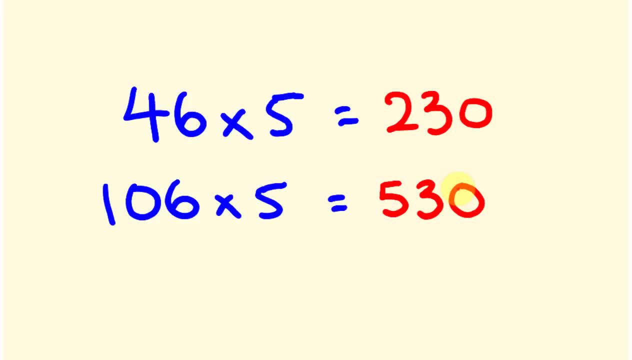 Okay, so the answer: 530.. Pretty basic, right? What about I give you one more of these? I'll show you the slight variation with this and I'll tell you why this works. So let's have a look at this. 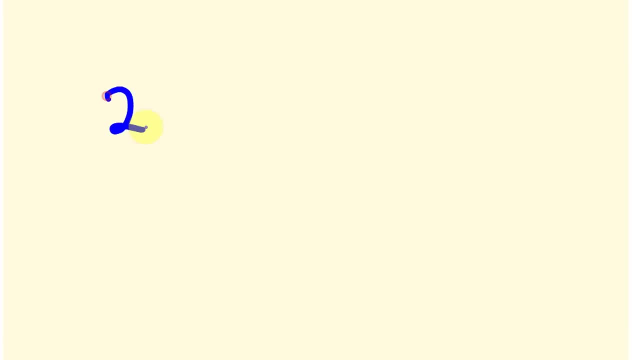 So say you had the following: one Slight variation might be a number that doesn't halve just as easily, which is 27 times 5.. Okay, it's, because half of 27 is not a nice even number. So all we're going to do is: 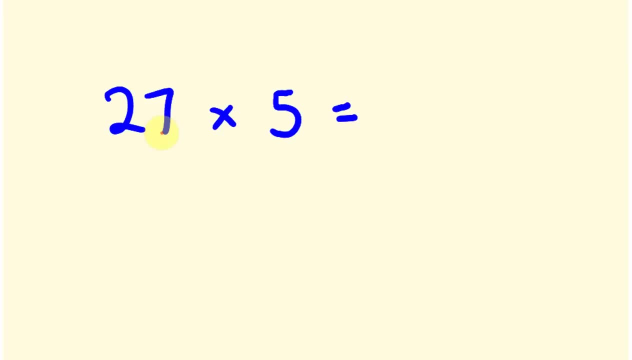 we're going to look at the number below this, which is 26,, and we're going to halve that number. Okay, so, half of 26,. well, that's 13.. And you're going to see that there's one lot of 5 left over. 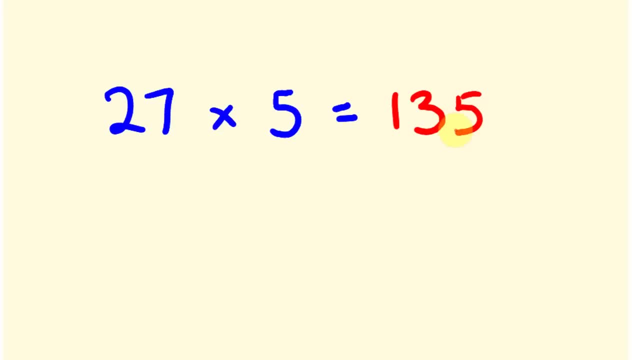 So that one lot of 5 left over. we're just going to add that on there, Okay, so the answer: 135.. So why does this work? Now, this is a really really easy idea to think of why this works when you think about it. 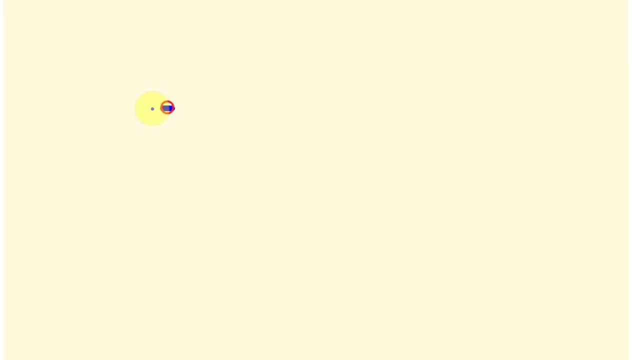 because, realistically, if we were to think about 5,, 5 is the same as saying 10 divided by 2.. Okay, so what we're doing is we're dividing by 2 first, and then we're just multiplying by 10, and that's why this works okay. 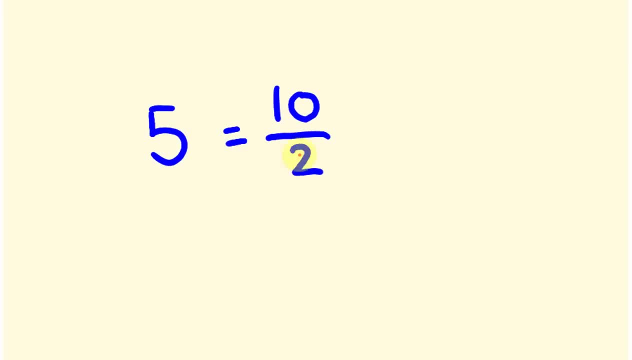 Because it's pretty much the same thing as we just got there. okay, We're dividing by 2 and timesing by 10.. Okay, what about I show you the 25s and how this works? okay, And look, I think you probably won't be that surprised once you get this started to get worked out. 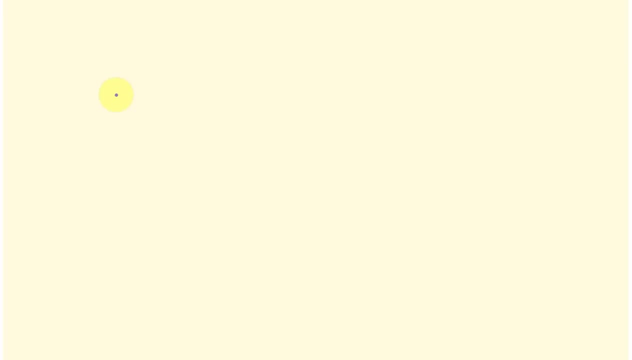 So say, we were working out with 25, and I wanted to know what 36 times 25 was. So straight away. hopefully you can look at this answer and you can say 36,. now we're going to be dividing not by 2, but by 4.. 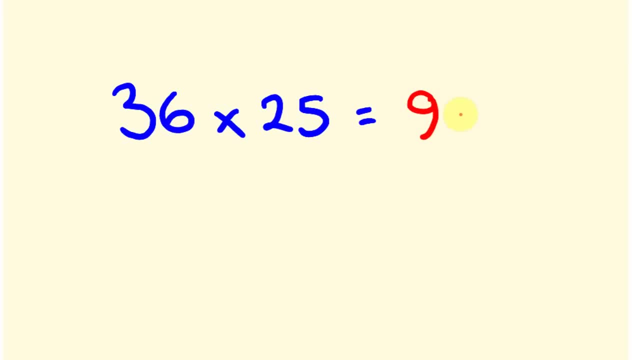 So 36 divided by 4 is 9, and we're going to be multiplying by 100,. okay, So when you're multiplying by 25, we're dividing by 4 and timesing by 100. Why is this? Because 25 is the same as okay 25,. I'll put this in a different colour. 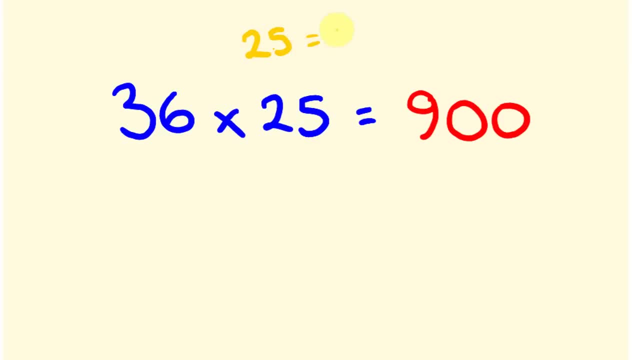 25 is the same as 100 divided by 4, okay, So what we're doing is we're now dividing by 4 and timesing by 100, okay, So we've been multiplying by 25, that's how you do that one, okay. 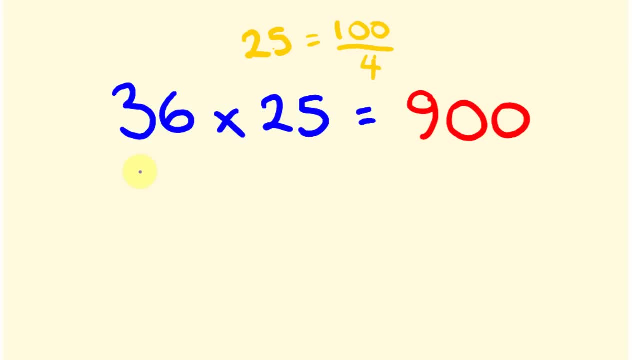 Well, what about we do another one? What about we do 64 times 25?? Okay, so what do we do? first, We divide by 4, so 64. Divided by 4, hopefully you're going to get the answer of 16.. 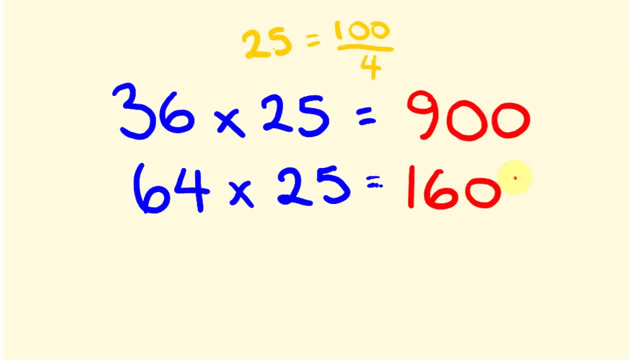 And we're just putting these two zeros, we're multiplying by 100.. Pretty easy, right? Hey, what about I just do one more of these a little bit harder? What about we do 17 times 25?? And the reason I've chosen 17 is because 17,, unlike these other ones. 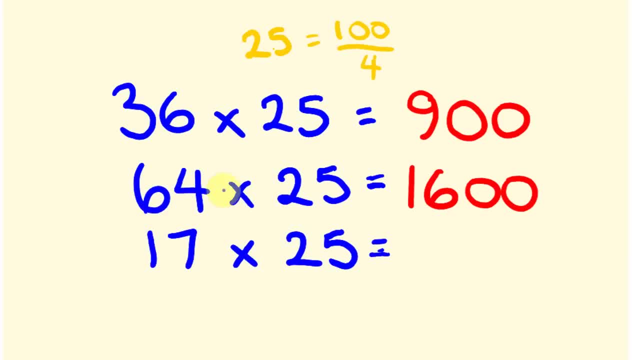 4 doesn't go nicely into it. Okay, I have purposely chosen these other ones to have 4 nicely. They don't necessarily go into them, but this one it doesn't. So we still do the same thing, We divide by 4, but we're looking at the number which is below this, that 4 goes into, which is 16.. 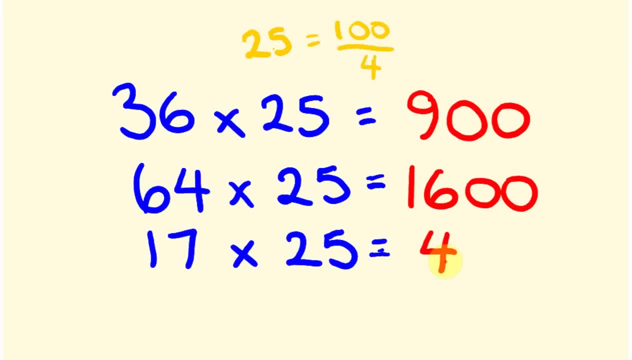 And that goes in 4 times and you're going to see there's 1 left over, So we're going to add this. So 25, okay, 425, no problem, right? That's how we do those, okay. 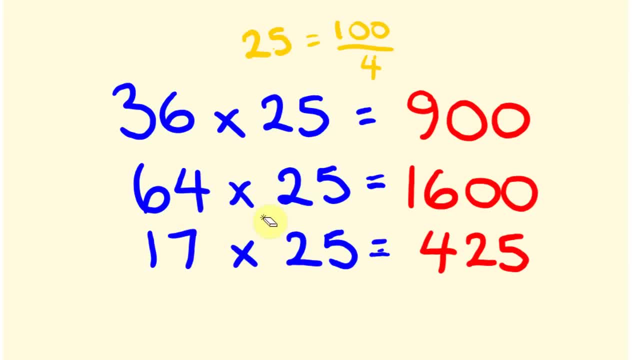 So we're just adding 1 group of 25.. If it was say 18,, we'd add 2 groups of 25.. If we were up to 19,, we'd add 16.. 3 groups of 25, so 75 to the answer. 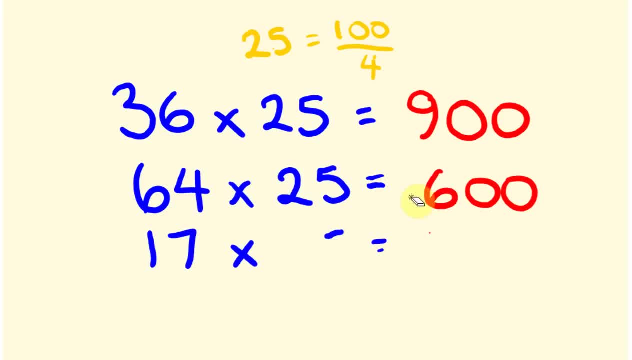 So you're sort of just going to keep that in your head, okay. Okay, what about the last part now which I said we're going to cover, Which is as follows: It's not rubbing out too quickly today, Okay, so say, we were looking at now multiplying a number by 125. 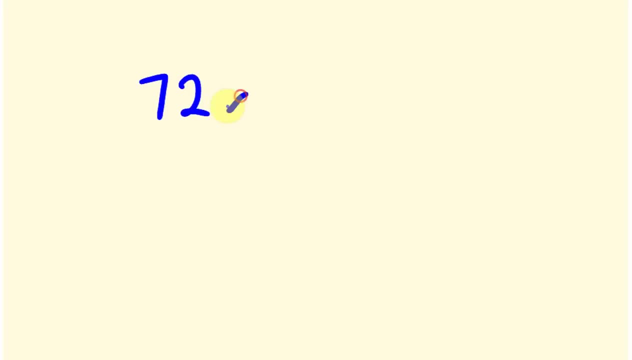 Say we had 72 times 125. Okay, well, before we start on that, we might think of 125 as being 1000 divided by 8, okay, You can see that 125 is 5 times 5 times 5.. 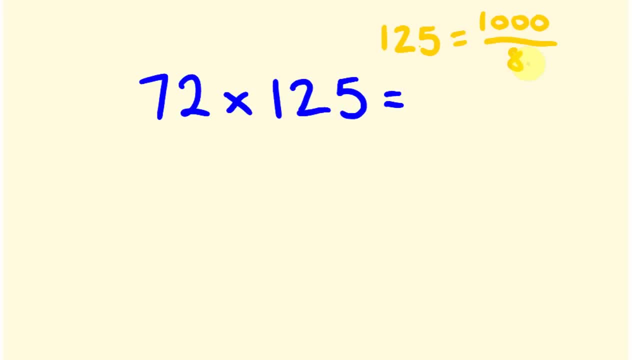 8 here is 2 times 2 times 2.. There's a bit of a relationship there, okay? So just to keep that in mind, if you might pick that up. But if we were multiplying by 125, now we're going to be dividing our number by 8,. 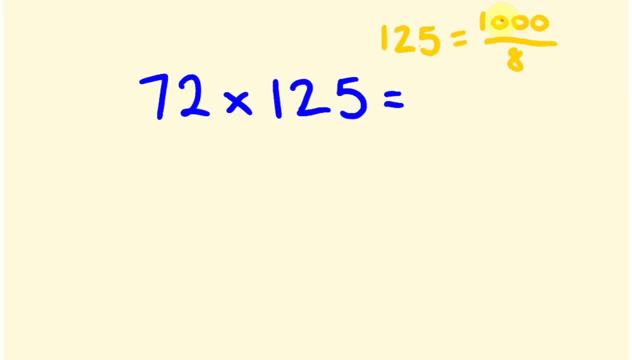 and then times it by 1000,. okay, So you can think of any number that you're multiplying by. You can actually change it to a fraction like this if it makes it easier for you. okay, So 72 times 125.. 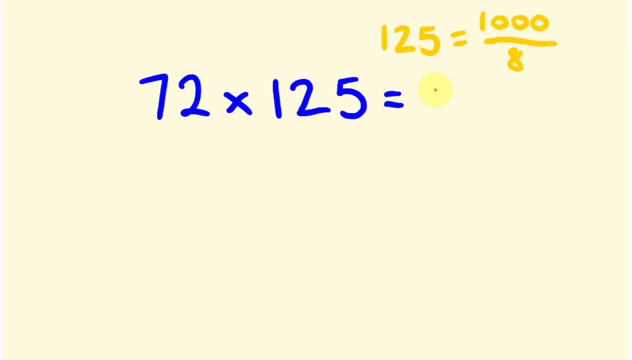 Okay, we can divide by 8.. So 72 divided by 8 is 9.. And we're going to multiply our number by 1000, 9000.. That's our answer. Okay, what about a bigger number now? 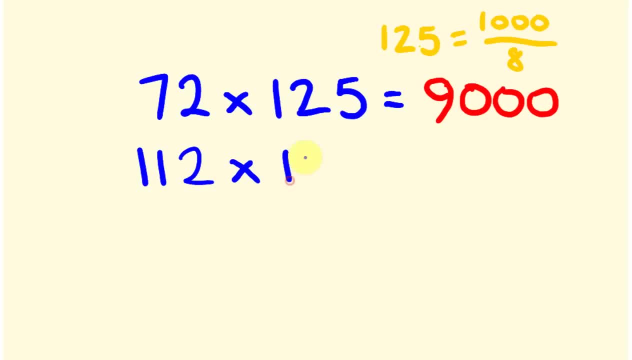 112 times 125.. Well, this doesn't seem to want to work, so we'll just write it there. Okay, what's our equal? Okay, So what are we going to do? We're going to divide our number here by 8.. 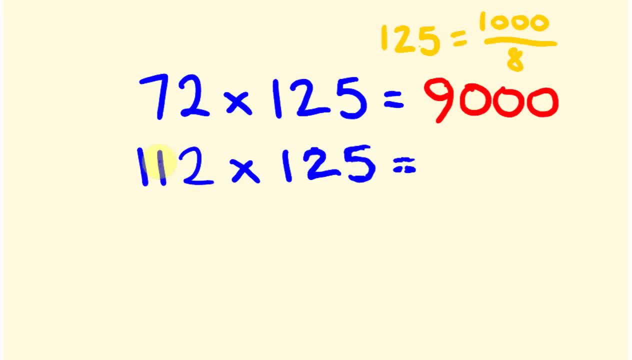 So let's do that. So 112 divided by 8.. Hopefully you're going to get the answer of wrong colour. It's sticking to the answer of 14. And we're going to put 2. 3 zeros on the end. 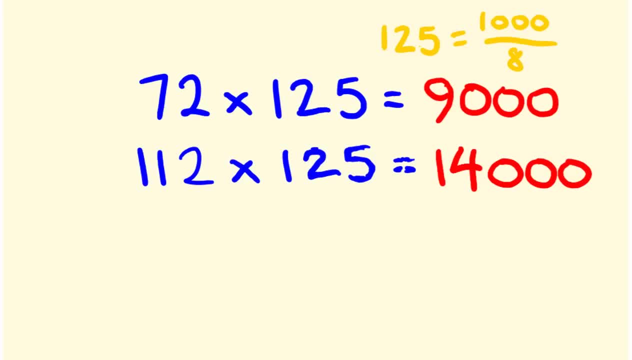 So 14000. Okay, Last of all, what about you know a slight variance here? What about we did 42 times 125 equals? Oh, that really bothers me. So I'm going to tidy it up by making it worse.